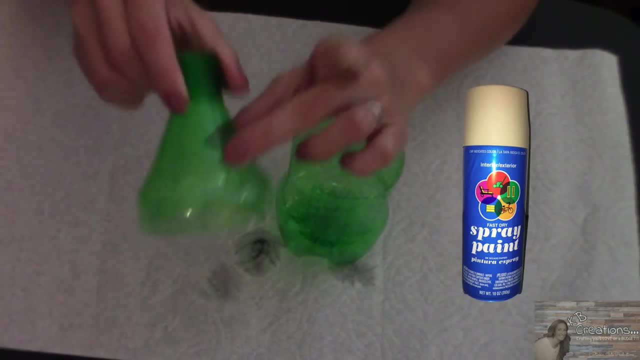 to spray paint the lid cream. I'm going to spray paint the top of the bottle red and I am going to spray paint the bottom red. I'm going to spray paint the top of the bottle green and I am going to spray paint the bottom. 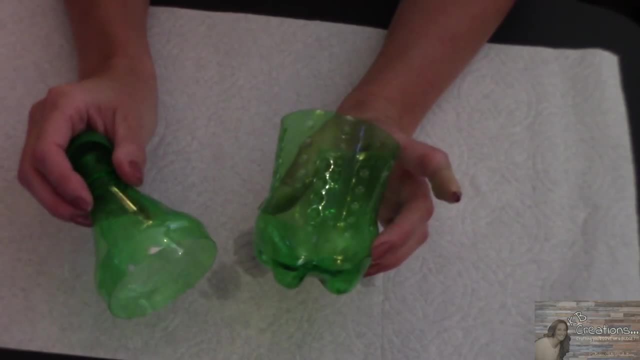 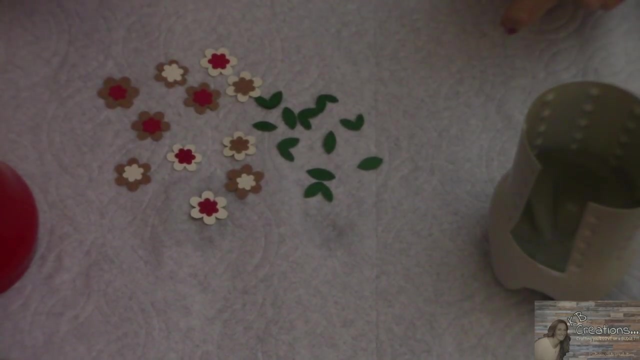 of the bottle cream and I am going to paint it and coat it until I have the coverage that I'm happy with. I've also cut out a bunch of small flowers on my cricket. You can paint and decorate this birdhouse if you'd like. I decided to cut out some cute flowers that coordinate. 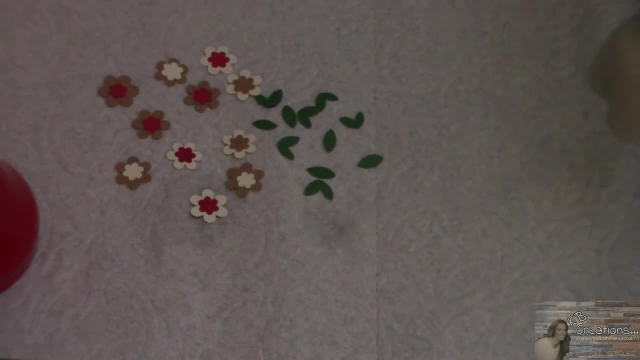 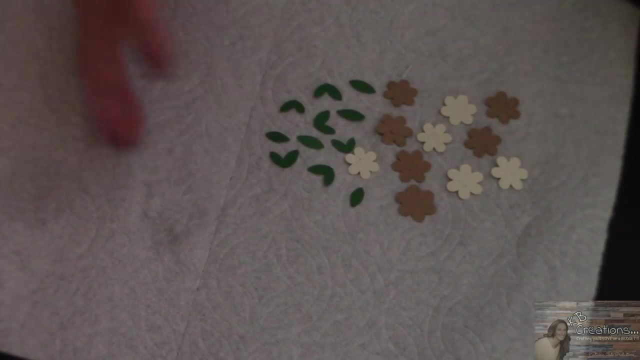 with the colors that I've painted it and I am going to use a Krylon spray adhesive to apply them. The flowers that I used are flowers that came up because I belong to the Cricket Club and I just picked out a cute flower that I liked, that had a cute leaf on it, and I did. 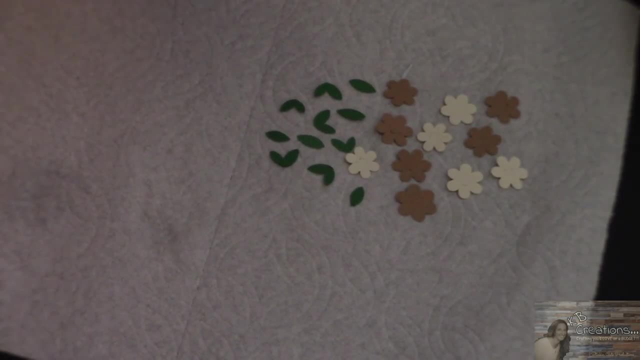 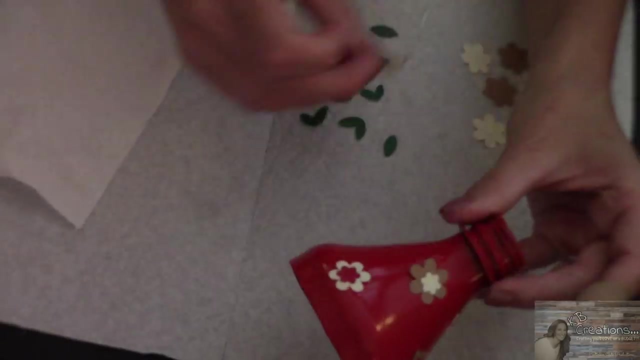 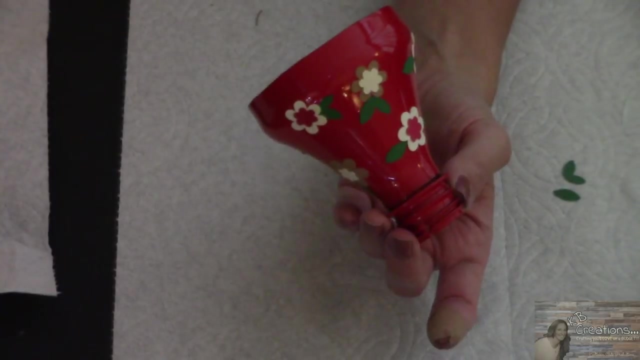 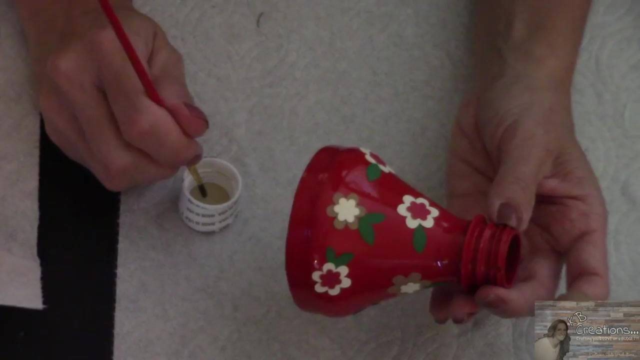 it down to about a quarter of an inch to a half an inch in diameter. I've applied all my flowers. Now I think I am going to take off the lid. I'm going to take some beige acrylic paint by Apple Barrel and I think I'm just going to add some dots. 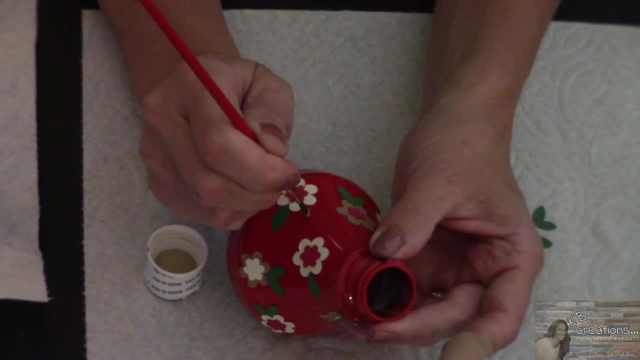 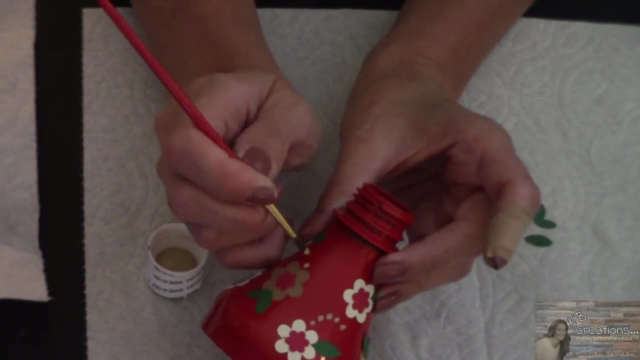 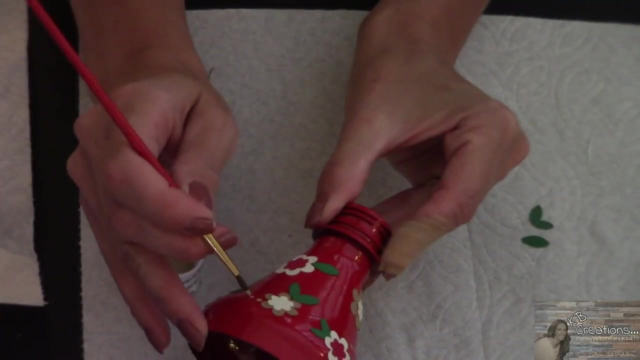 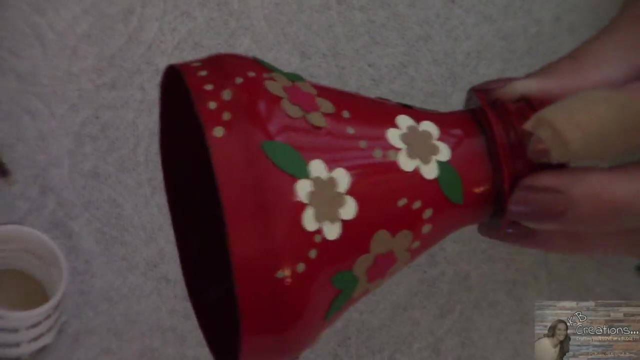 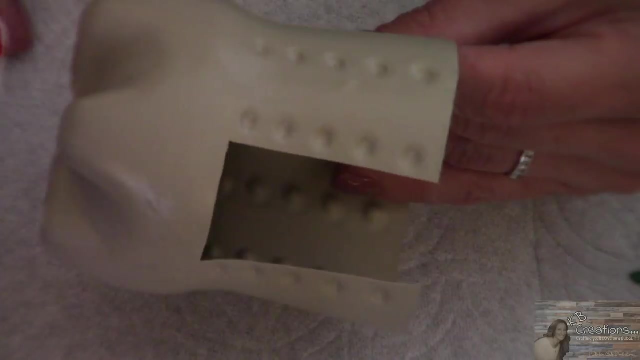 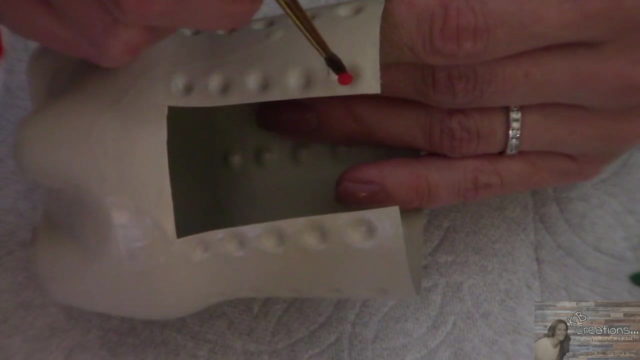 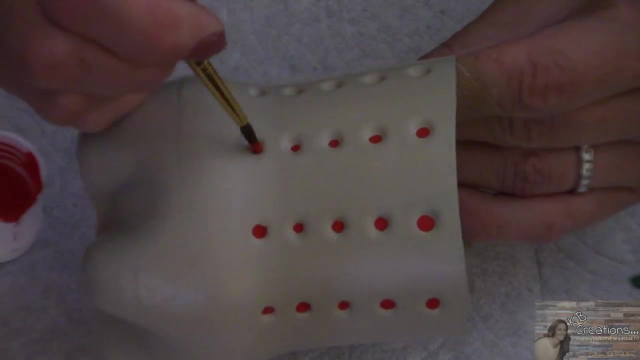 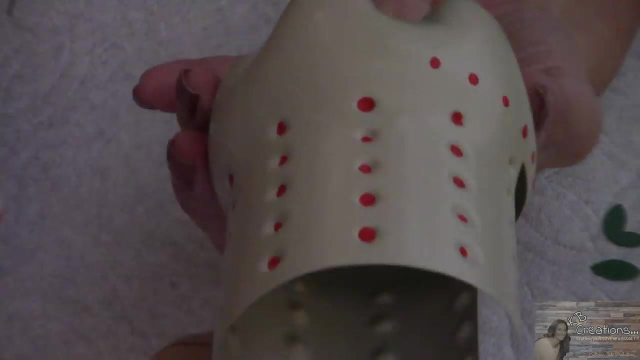 to dress it up a bit. Now I'm going to take the bottom part of my bottle and I'm going to decorate it as well, And the Sprite bottle makes it easy- because you've got all of these indentations already- that you can just put dots in. 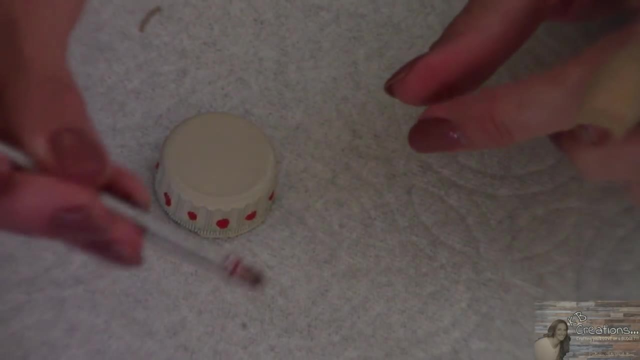 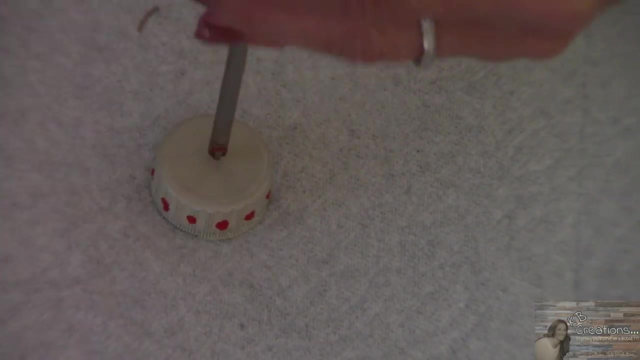 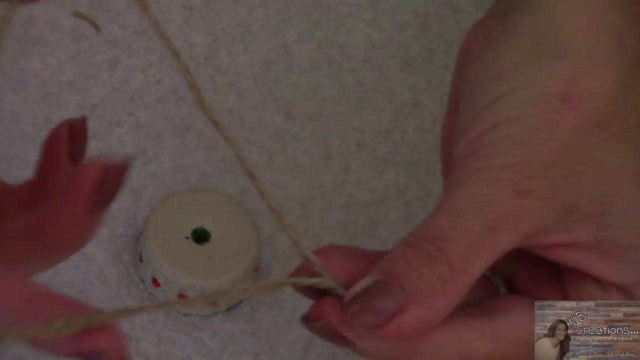 We are going to take our Sprite lid, we're going to take a screwdriver and we are going to hammer a hole in the top. Okay, Okay, Okay, Okay. Then we're going to take a piece of twine and our lid is done. 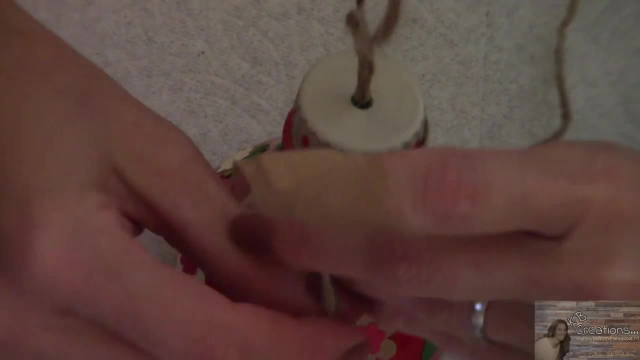 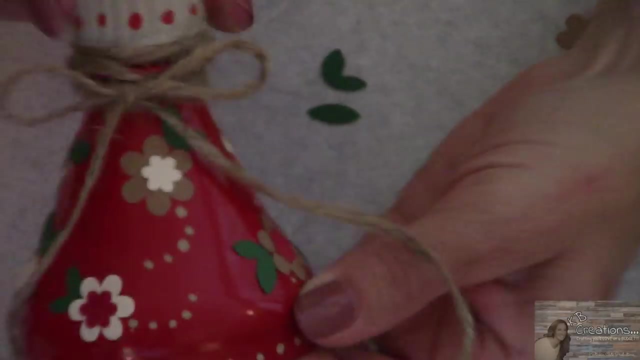 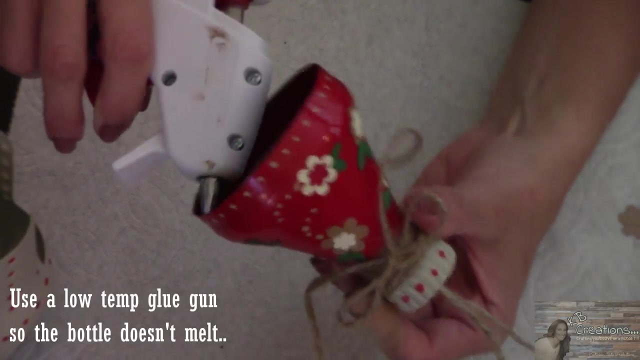 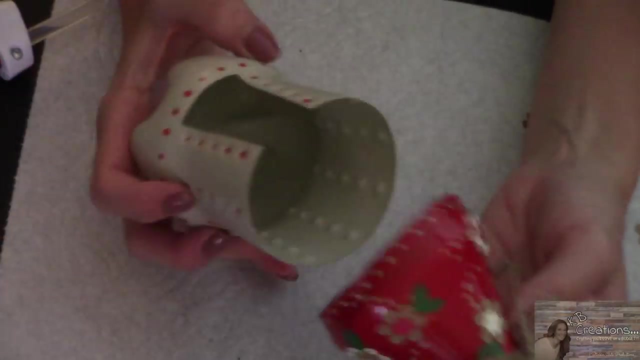 I'm going to take some twine and I am going to wrap it around the neck of the bottle here. Then we're going to take the top of our lid and our hot glue gun and we are going to put hot glue on the inside about three quarters of the way around. 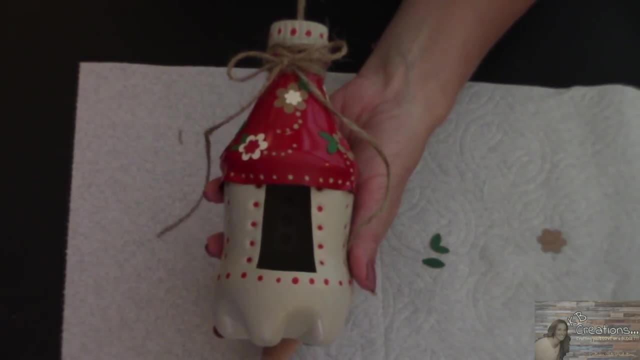 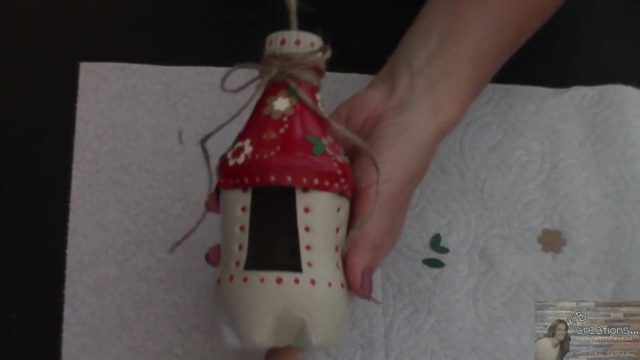 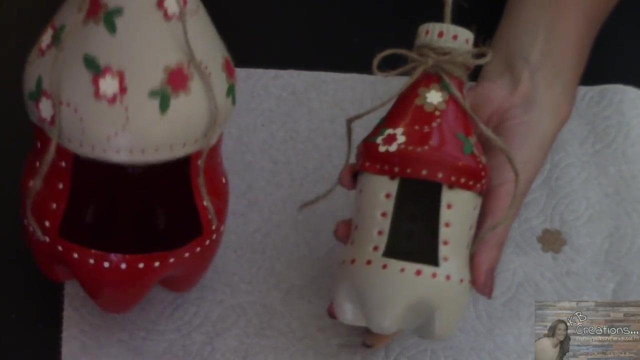 And there you have it, our bird feeder or birdhouse made from recycled soda bottles. Isn't that adorable? And if you want to make a bigger birdhouse, I made a coordinating one out of a two liter bottle Sprite bottle that you can make and that makes it an even bigger birdhouse. 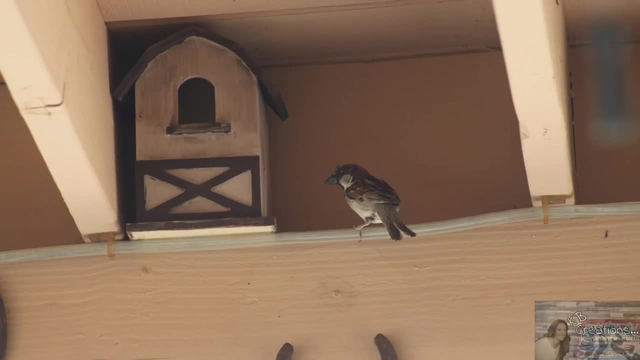 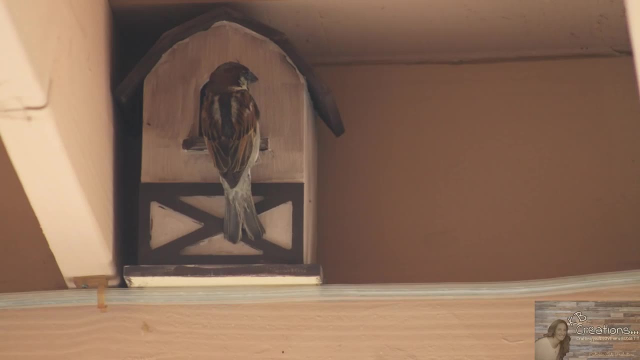 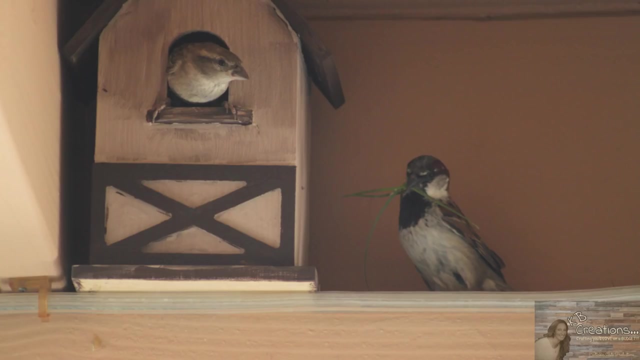 We have birds that come back to us. They come back to our house every year around this time and a few years back we went and bought the wood birdhouses that Joann's and Michael's made and we each decorated and painted one of the birdhouses and, honestly, the birds made beds in them and put grass and hay and 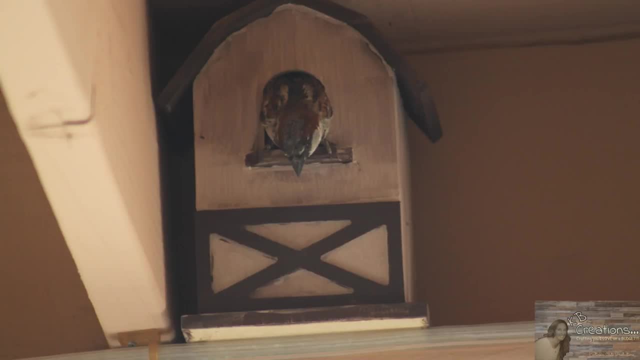 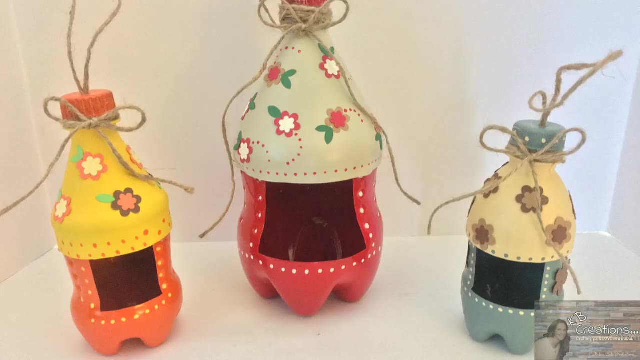 leaves in there and they come back every year. Well, everybody, that's all I have for you for today, for this DIY birdhouse Bird feeder made from a recycled Sprite bottle. I hope you enjoyed this video. Please give it a thumbs up if you liked it and if you're new to my channel, stick around. 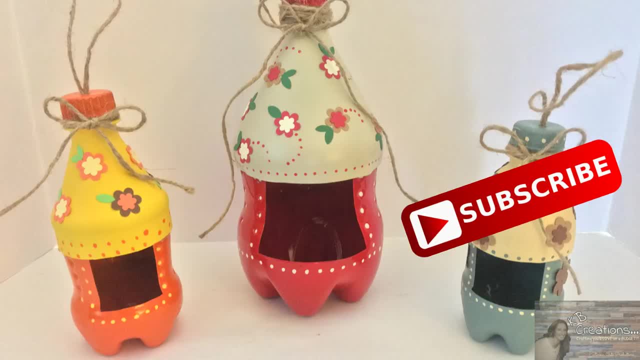 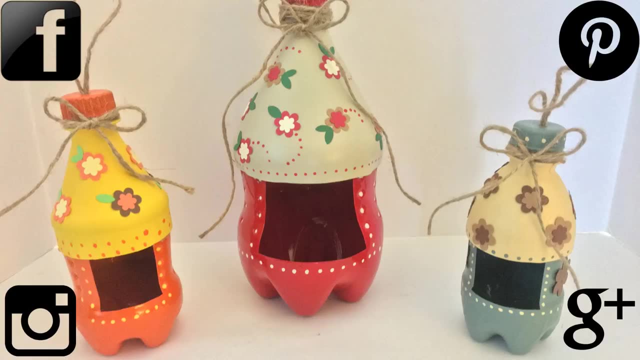 a while by clicking that red button for more crafting on a budget. more everything on a budget: videos to come. If you click it again when the bell appears, YouTube will notify you when I'm uploading a new video. You can also follow me on Facebook, Pinterest, Instagram and Google Plus. 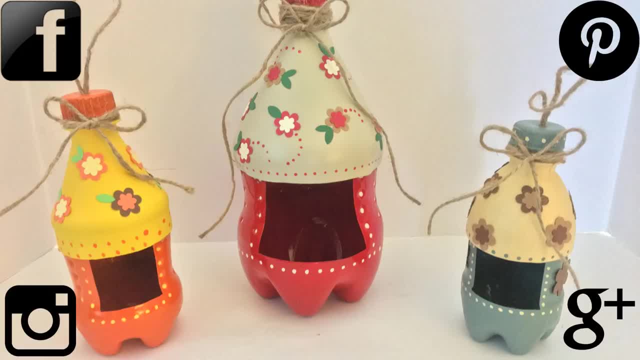 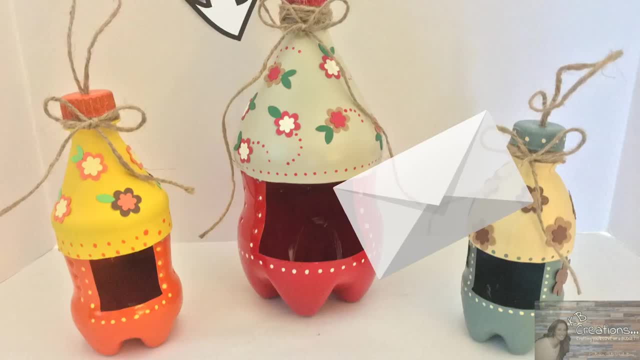 Those links are in the description box below. Just click on the link If you like those links. click, follow, and you'll also be notified through social media when I'm uploading a new video or just doing something fun. You can also find my PO box in the description box below as well if you're interested in. 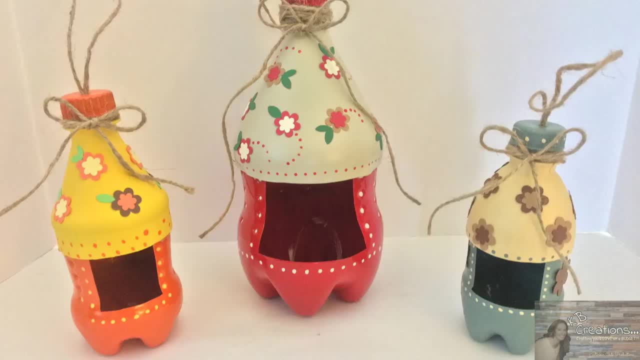 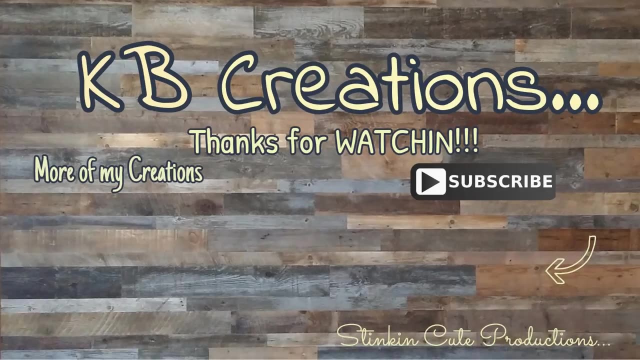 sending me fan mail and watching me open it up in a video. Until next time, everybody, I hope you have a fantastic day, Happy crafting on a budget and bye for now. Bye for now.